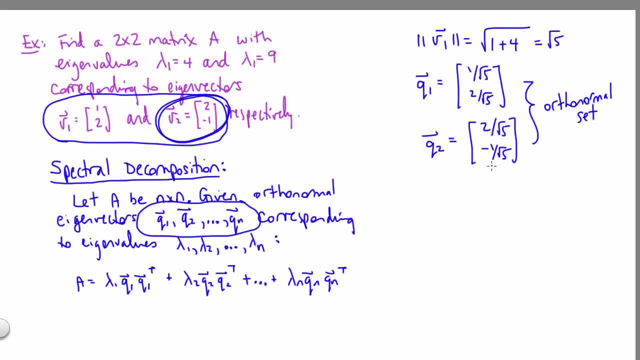 do each have length 1.. So now we have the conditions of the spectral decomposition satisfied. We're working with this. 2 by 2 matrix A, so we're going to be able to build A using this sum here. So A will look like lambda 1 times q1. 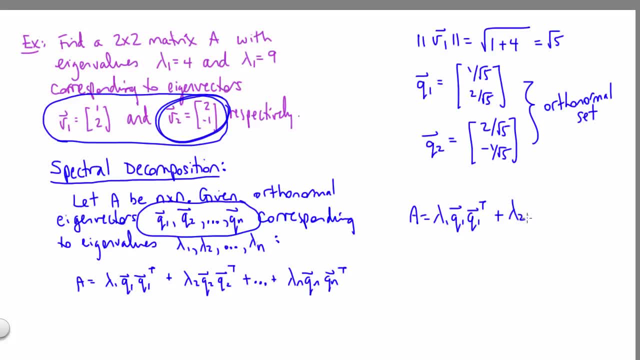 times q1 transpose, plus lambda 2 times q2 times q2 transpose. So, making this more specific, lambda 1 is 4 and lambda 2 is 9, so we'll be able to plug in these values as well. Now I've. 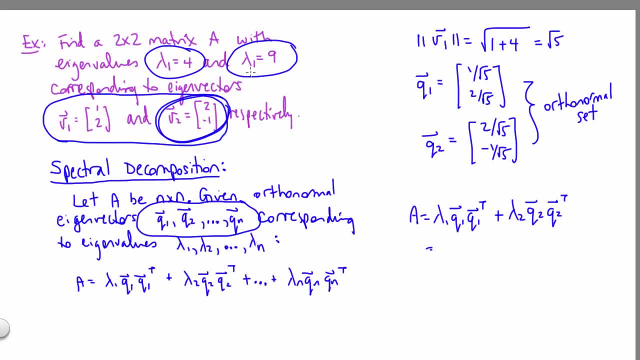 just noticed that I made a little bit of an error in writing down the question. This should read: lambda 1 is equal to 4 and lambda 2 is equal to 9.. So hopefully that didn't cause too much confusion there. Lambda 2 is 9, that corresponds. 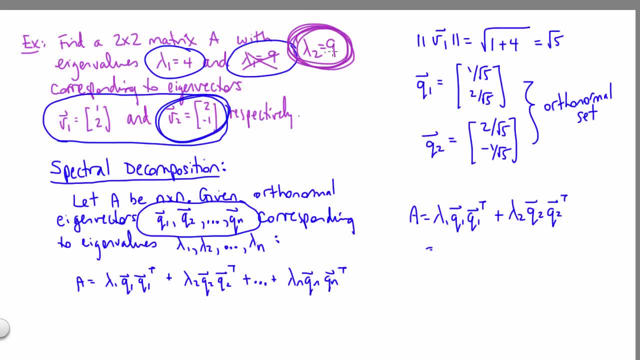 to the eigenvector v2.. Alright, so now, with that correction made, we should be able to plug in to our expression down here: for A, 1 is 4.. q1, looking up here looks like 1 over root 5. 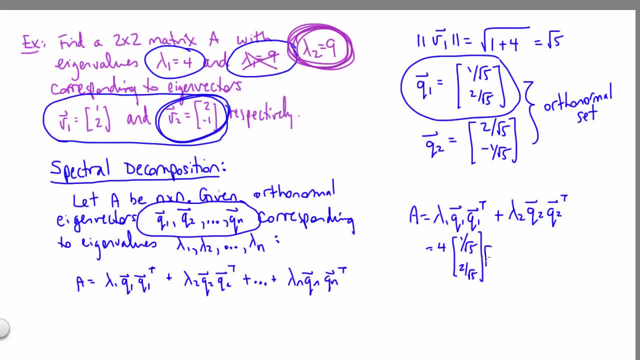 2 over root 5, and we're going to multiply that by its transpose And we're going to run out of room, but we just managed to squeeze it in there, Alright. so let's continue with our calculation. I'm going to work on. 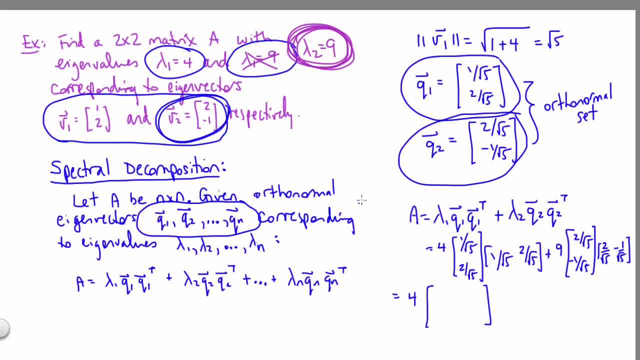 this matrix multiplication here, As we multiply through, we're going to have 1- 5th, 2 5ths, 2 5ths and 4- 5ths, And that 4 will stay out in front, And then we've got. 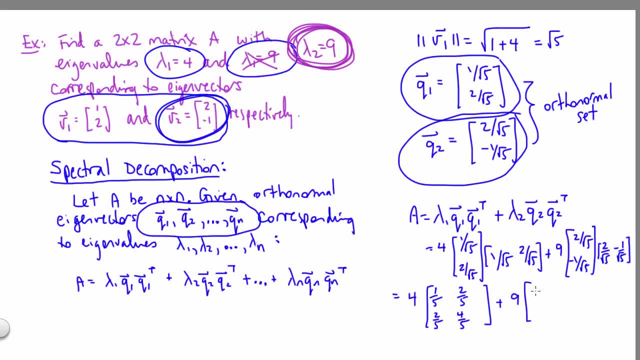 plus 9 times 4 5ths minus 2 5ths minus 2 5ths and 1 5th, And we'll do just a little bit more algebra here to get a final answer for A. So I'll leave the question written up here and let's continue.